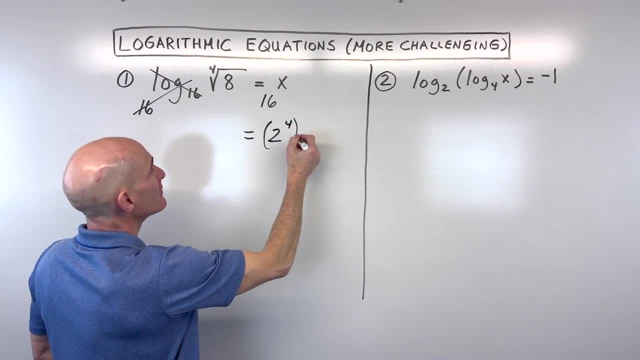 do here is 16 to the x. power equals the fourth root of 8.. And so what we're going to do here is is actually like 2 to the 4th power, 8 is 2 to the 3rd power, and then this is the 4th. 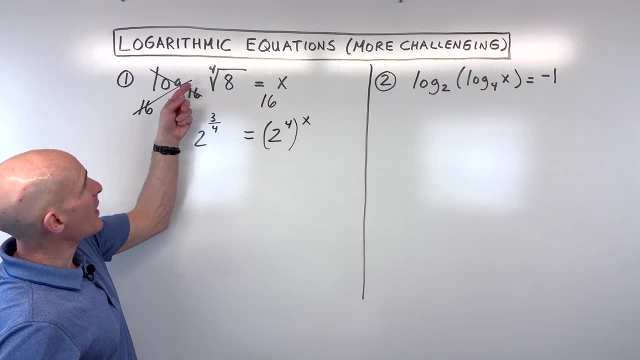 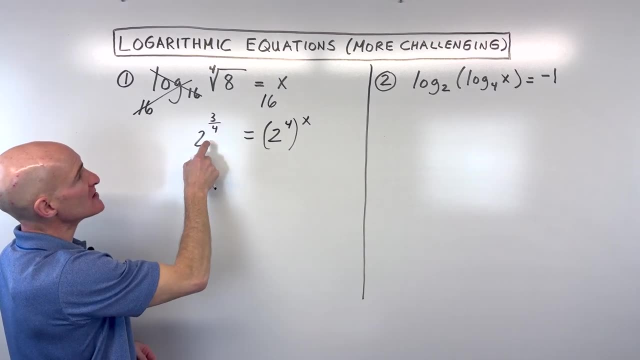 root. So here we're talking about rational exponents. Remember rational exponents. this index or root goes in the denominator and the numerator. the exponent is the power. So you can see, 2 cubed is 8, and then we've got the 4th root of that. Now remember when. 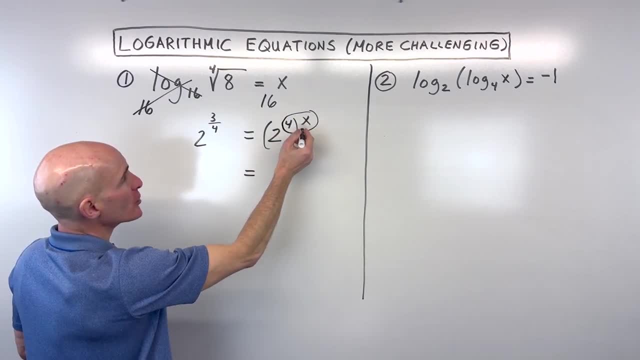 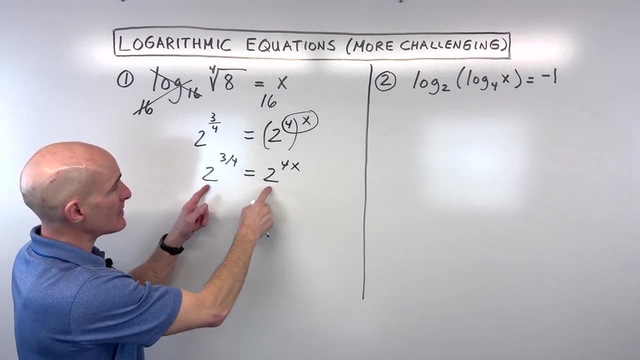 you have an exponent raised to an exponent, or we call it a power to a power. you multiply those exponents together and then now look what we have. We have the 1 to 1 property of exponents. We have the same base, so we can set those exponents equal to each other. 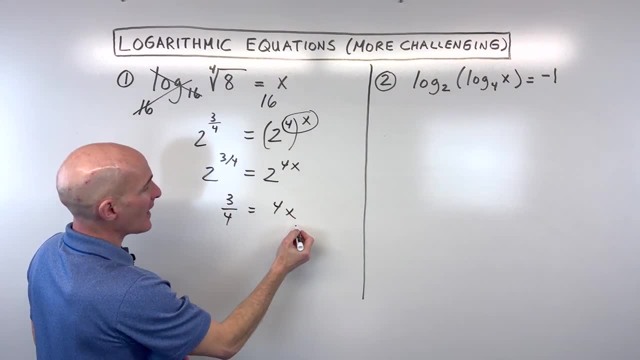 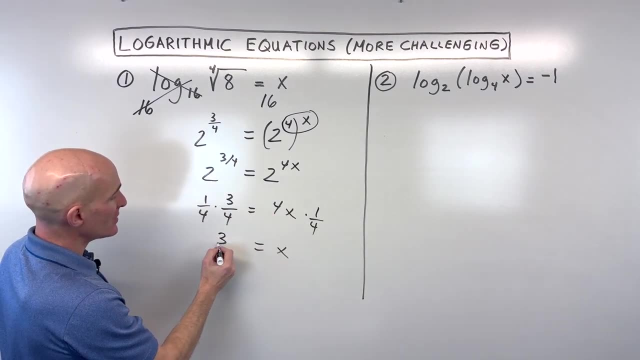 and solve. So we have 3 4ths equals 4x. Let's just go ahead and multiply both sides by 1, 4th and that comes out to x is equal to 3 16ths. With logarithmic equations you always. 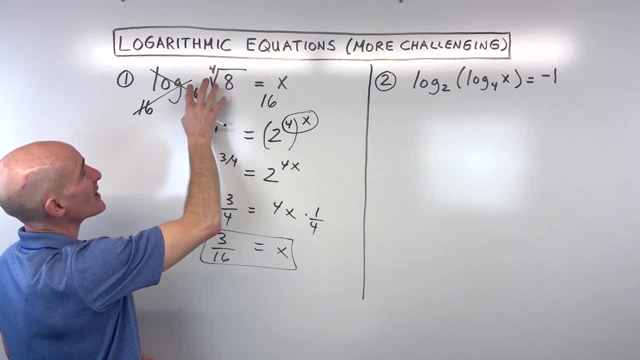 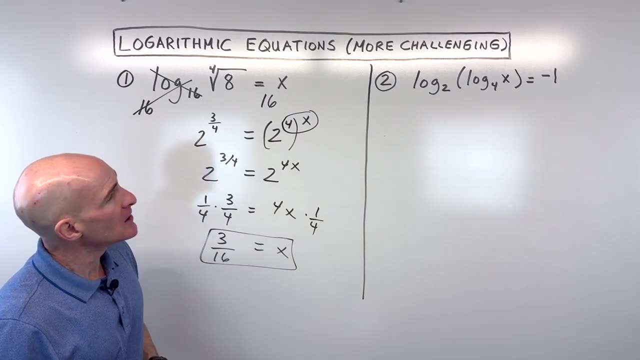 want to go back and just quickly check to make sure that you're not taking the log of a 0 or a 9.. That's a negative quantity, but that's not the case here. So let's look at number 2 now. 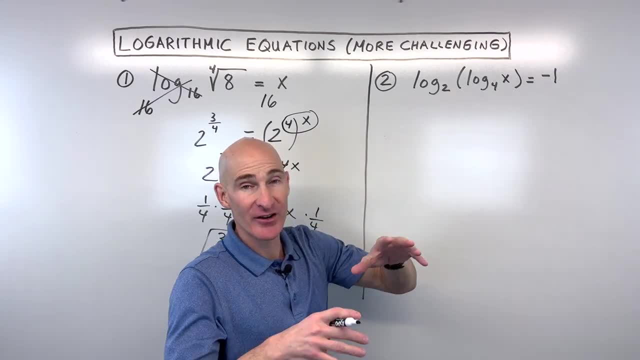 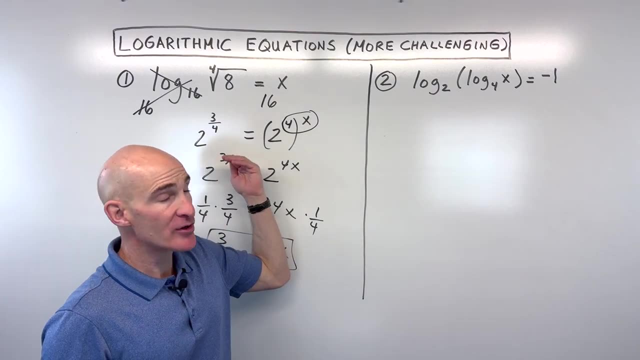 So here this is kind of interesting because we have like a log inside of another log. So how would you solve that one? Well, if I was going to do it, I would do very similar to this first problem, where I'm going to exponentiate or raise both sides or rewrite this in the 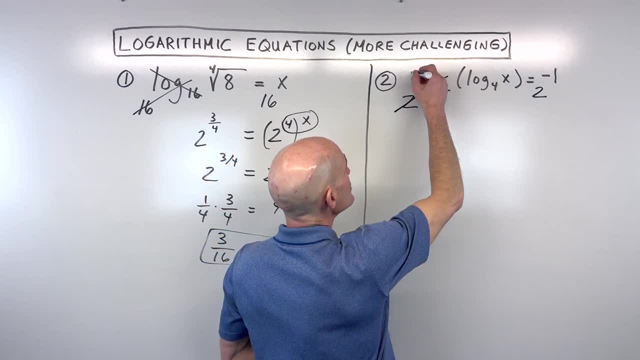 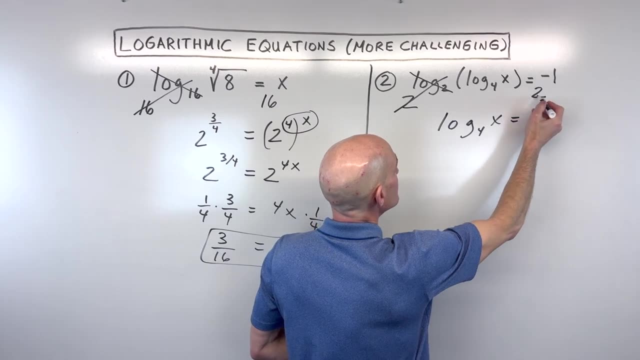 exponential form. however you want to think about that, These are inverses of one another, just like squaring and square, rooting, or adding and subtracting, multiplying and dividing, And so you can see we're left with 2 to the negative 1, which remember when you have. 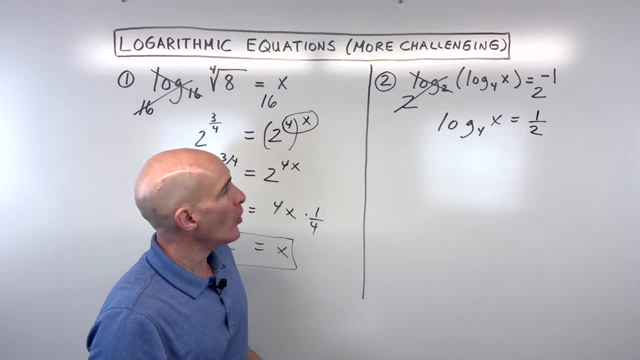 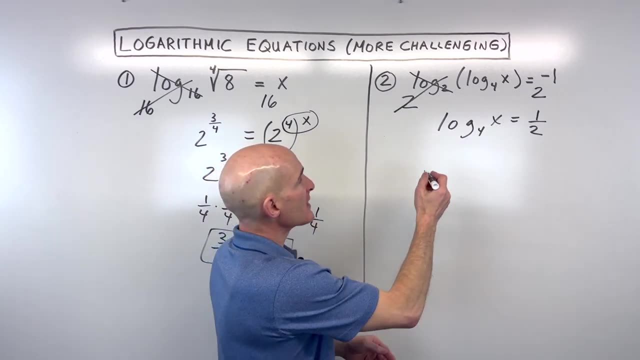 a negative exponent that tells us to take the reciprocal. Okay, so now we just have one log here, but again we're still trying to get that variable by itself. Let's do this one more time. Let's exponentiate both sides using base 4.. These are inverses. they undo. 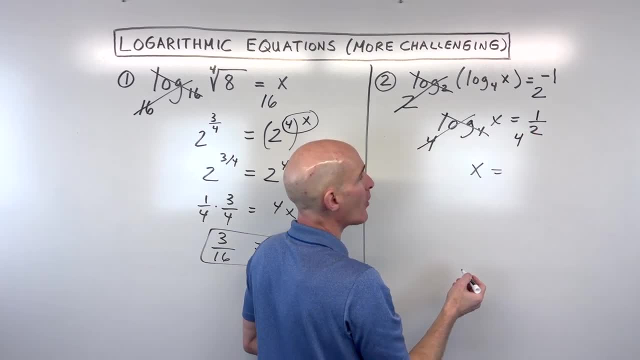 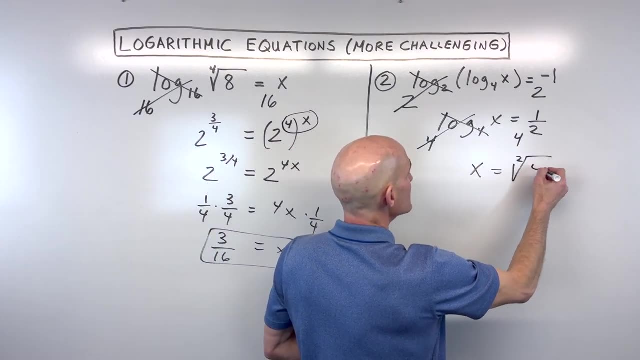 one another and we have: x is equal to 4 to the 1 half power. But remember, the 1 half power is the same as the square root, right? Because this is a denominator, that's our index. So this is like the square root of 4 to the first power. The square root of 4 is 2, and 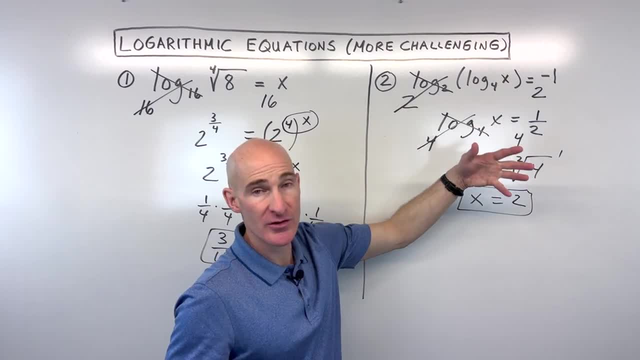 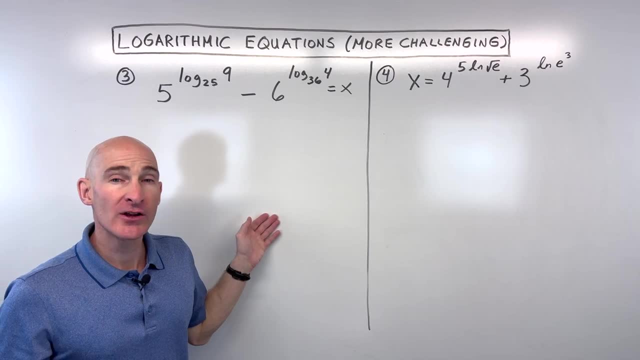 that's our final result. Again, you want to check to make sure you're not taking the log of 0 or a negative quantity, and in this case we're not. so this is a good answer. Let's take a look at two more examples. Okay, let's take a look at number 3 now. So we've got. 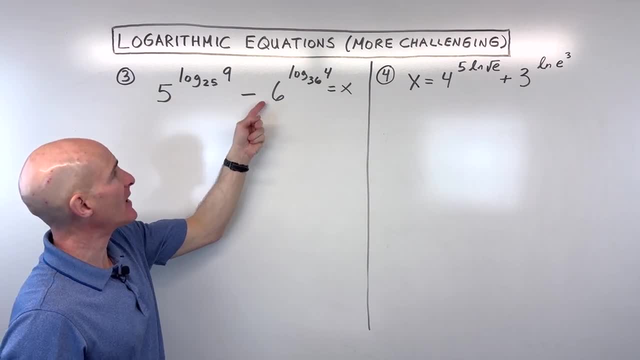 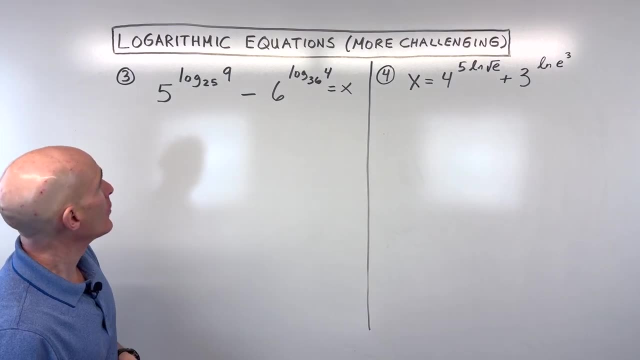 5 raised to the log base, 25 of 9 minus 6 raised to the log base, 36 of 4 equals x. How would you solve for x in this problem? Well, this is a challenging one, but notice that we've got 25 and 5.. That seems to be. 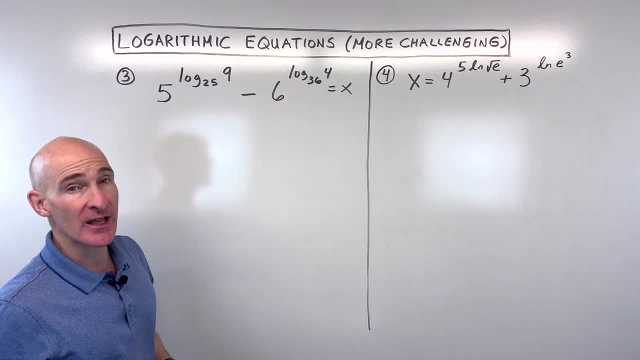 very interesting. We've got 36 and 6, that seems to be very interesting. Let's do a little bit of rewriting here. 5, we can write that as 25 to the 1 half power, right, Because the 1 half power is like the square root, and the square root of 25 is 5.. So we're not 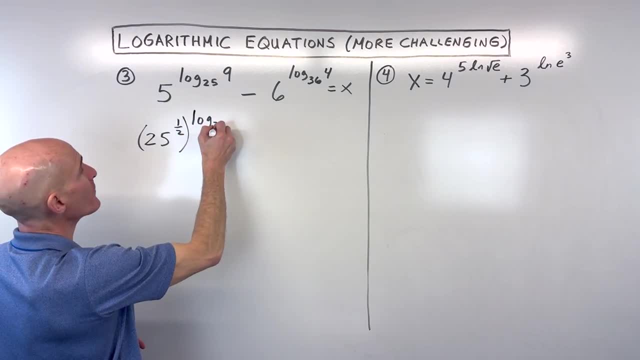 changing the problem. we're just rewriting it and putting it into a different format. Now over here. 36 to the 1 half power. Indeed, we have 1 half power, ie it's the half power of the square root, but the square root of the square root is also a half. 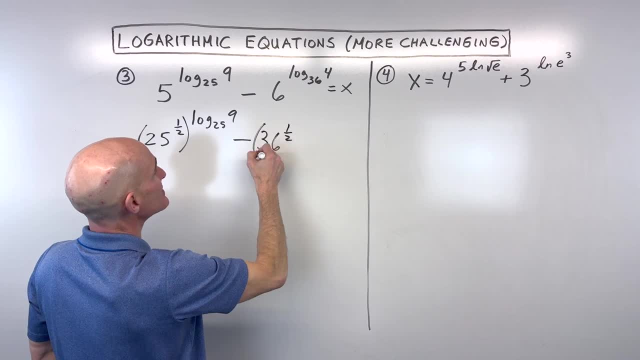 power. So i'm not telling you that this is a square root of the square root, so it's a square to the 1 half. power is the same thing as 6, because the square root of 36 is 6. And you're probably 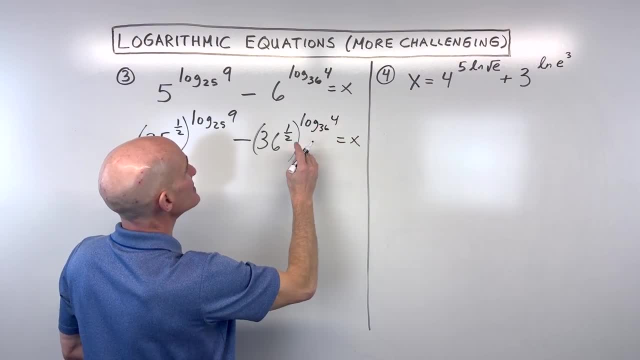 saying: well, why are we doing that? And you'll see in just a moment. here we're trying to get these bases to be the same. But now let's take a look at this Power to a power. what do we do? 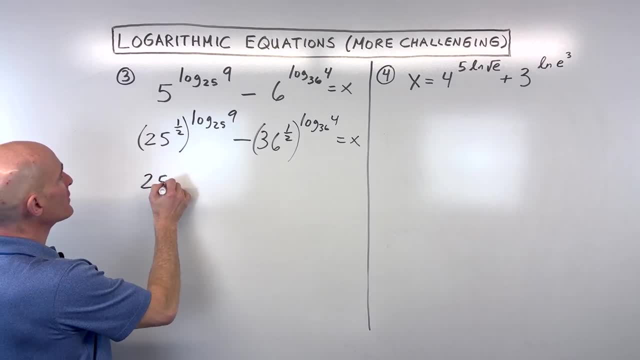 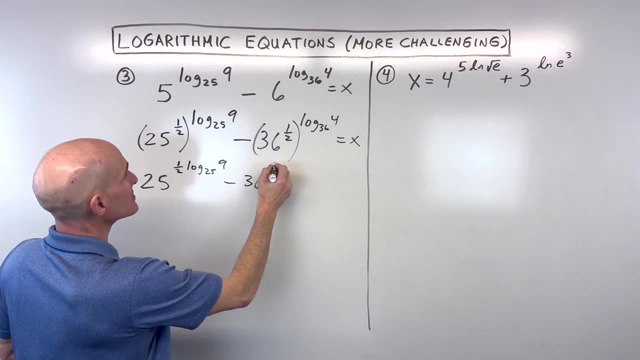 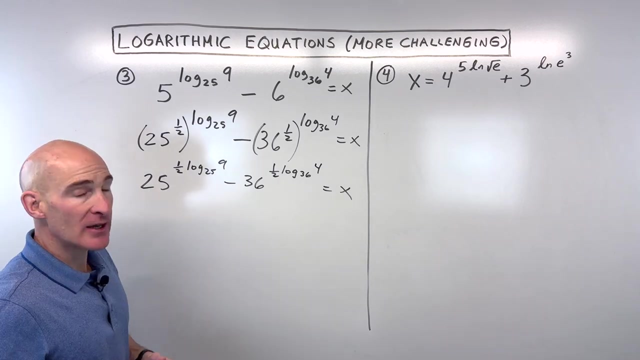 We multiply the exponents, So that's going to look like 25 to the 1 half times log base 25 of 9 minus 36 to the 1 half times log base 36 of 4.. Okay, now let's take a look at the. 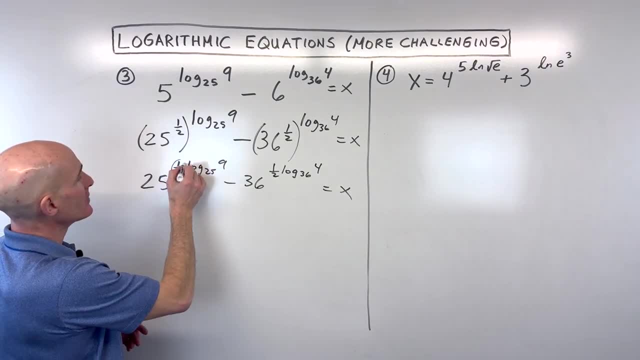 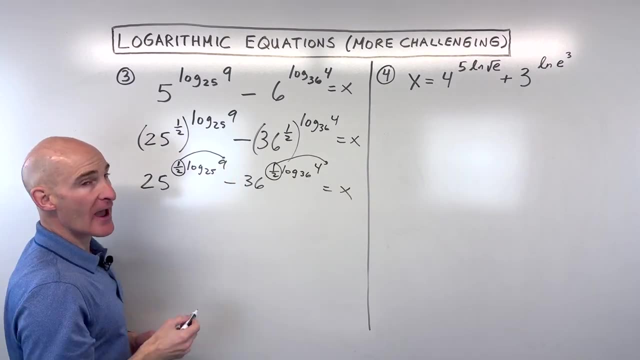 power. property of log. So whatever's in front here you can bring it up as a power. Same thing here: Whatever's in front we're going to bring up as a power. So now, when I think of 9 to the 1 half power, again that 1 half power is the square root. So that's saying like the square. 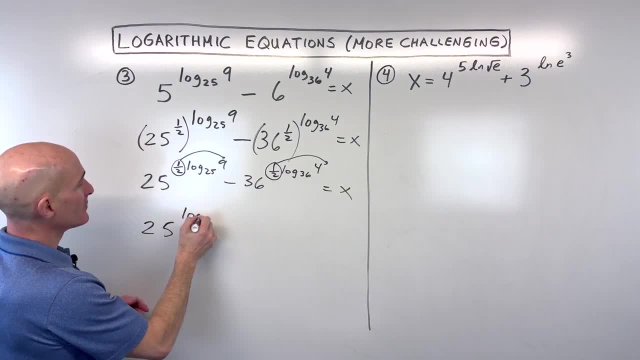 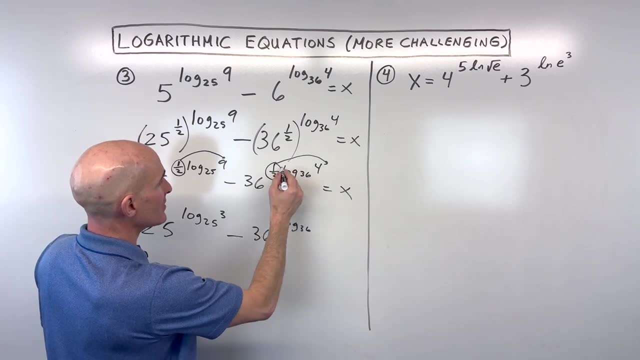 to 9,, which is 3.. So this comes out to 25 log base 25 of 3.. 3 minus 36 log base 36 of the square root of 4, which is 2.. Okay, so now look what we have We. 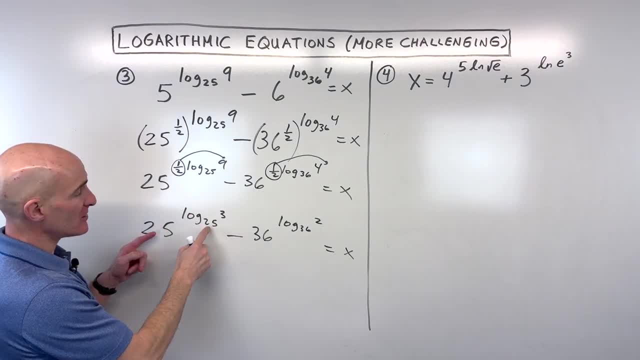 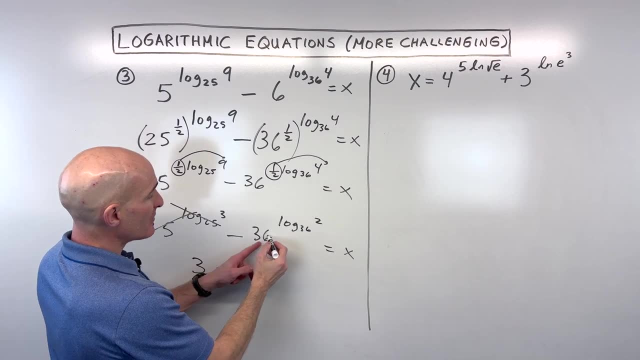 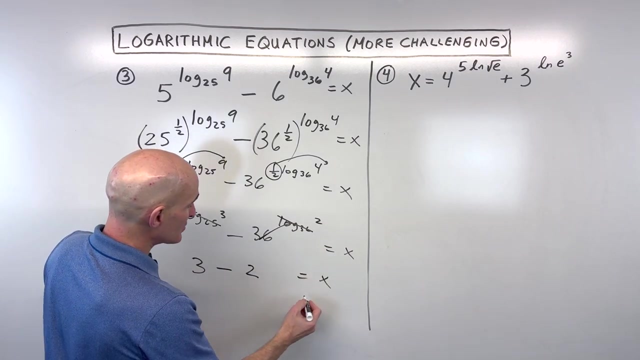 have an exponential function, We have a logarithmic function. The bases are the same. These are inverses. They undo one another. That leaves us with 3,. right Over here, same thing. We have 36 raised to the log base, 36.. These are inverses And we just get 2.. And 3 minus 2,. 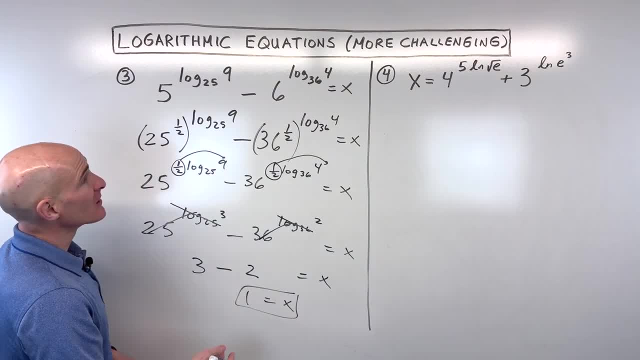 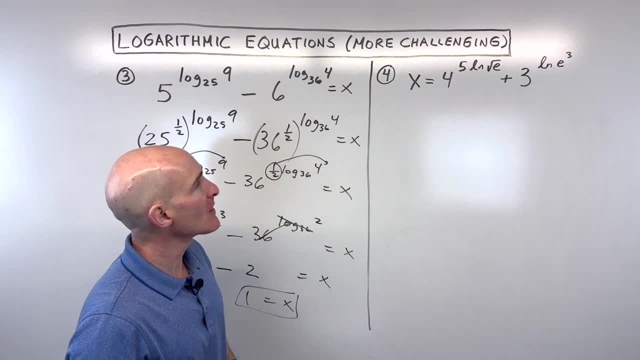 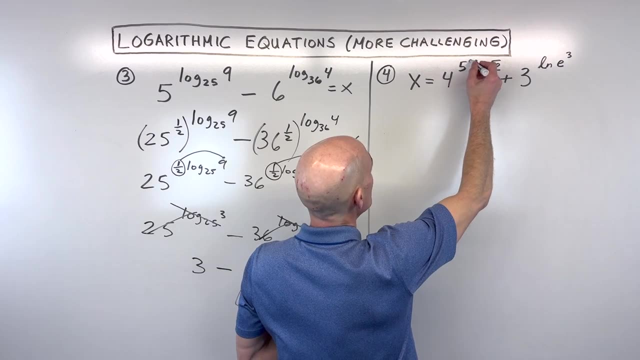 some natural logs here in this problem. How would you do this one? Well, again, we're going to want to try to rewrite this a little bit, And so what I would do is I would take this coefficient, bring it up as a power, That's the power property of logs, or natural logs, And so if we do that, 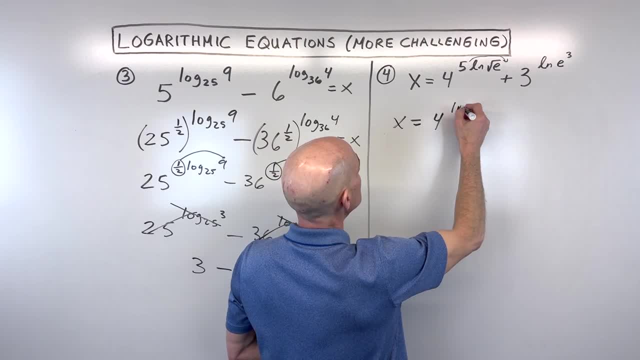 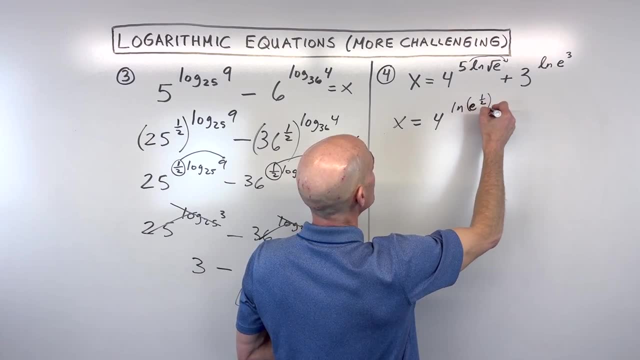 this looks like: x equals 4 to the natural log of now. c squared of e is the 1 half, right, So 1 half. But then we're bringing up this power like that. OK, so now we've got power, to power We're. 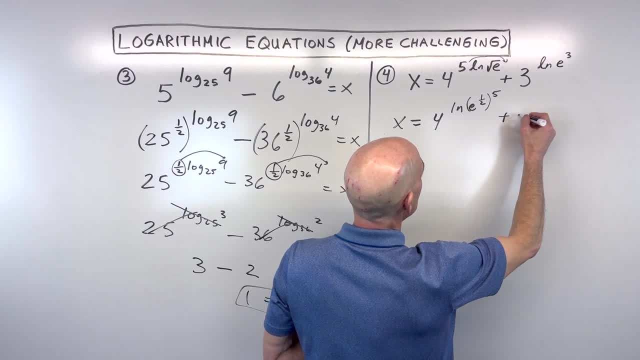 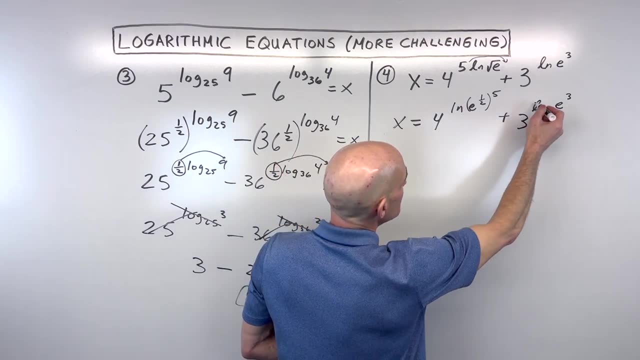 going to multiply. Let's simplify this a little bit further here. So this one, we have natural log, which remember. natural log is base e log, base e of e cubed. These are inverses of one another because the bases are the same And we just get 3 here. So this is really like 3 to the 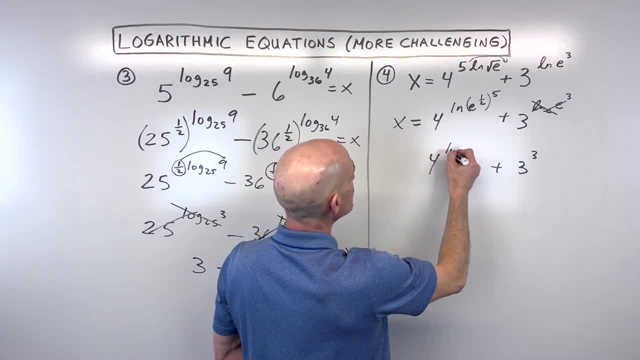 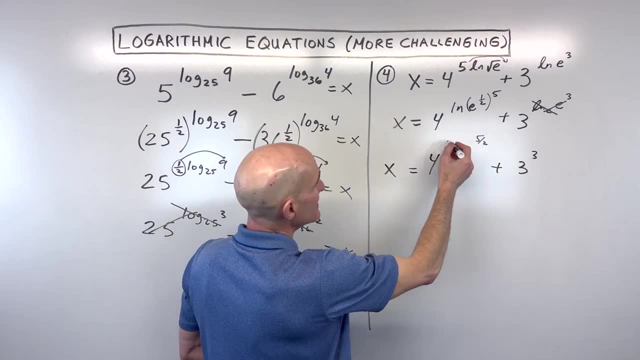 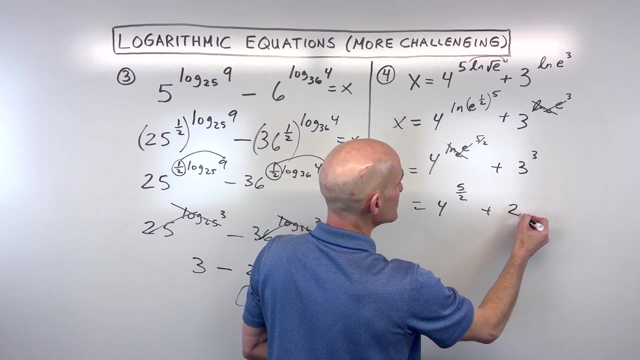 third power: Here we have 4 to the natural log of e, to the 5 halves power, Of course. remember, natural log is log base e And you can see that these are inverses of one another, leaving us with 4 to the 5 halves power, plus 3 cubed, which is 3 times 3 times 3,, 3 times right, And then this: 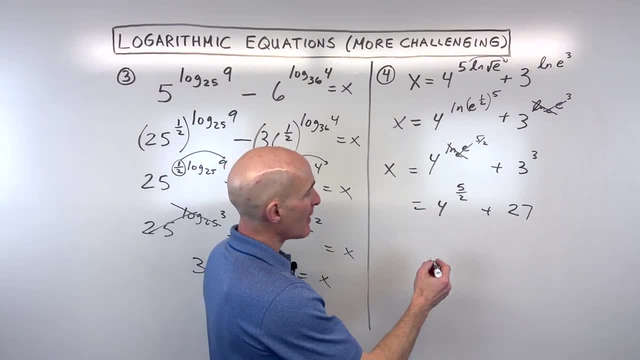 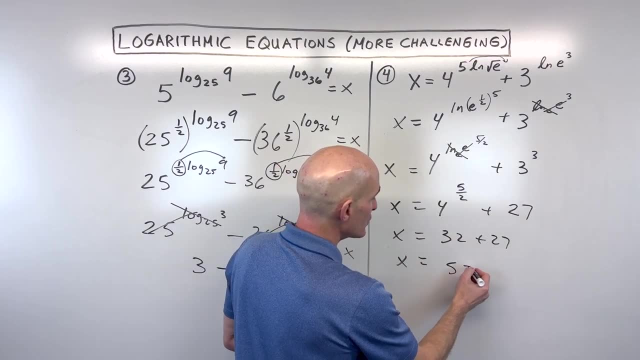 is saying: what's the square root of 4?? That's 2.. What's 2 to the fifth power? That's 32.. And now we just have 32 plus 27,, which is 59. And we solved it. So great job, if you're able. 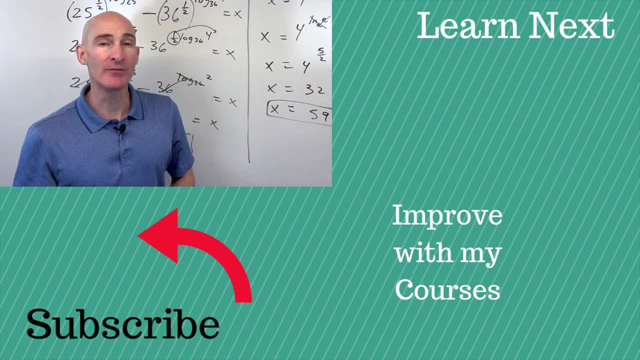 to follow these four For more challenging logarithmic equation problems. if you want to learn more about logarithms, I've got a complete guide right there. Follow me over to that video. We'll go through all the properties of logs: expanding, condensing logs, solving logarithmic equations.